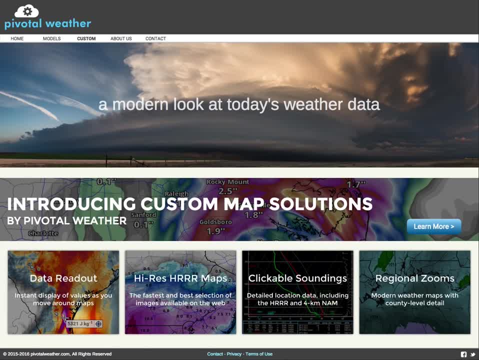 Dude Dudette, see if you've made it to the ultimate Pivotal Weather Models 101 series here. okay, And in this episode I'm going to talk about how you can use this, all the resources on here- like a professional weather forecaster would, And it's going to be easy. Anyone can do it. 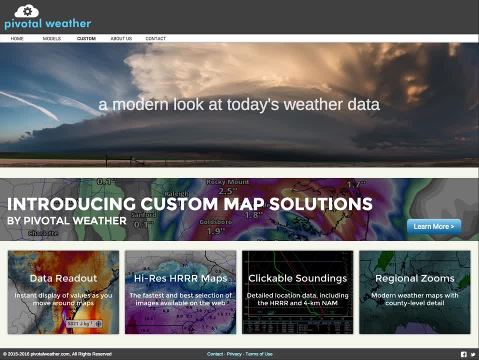 Anyone can do it, okay, And so I'm going to talk to you about the different types of models that we can use on here, the tools that you can use on here, and I'm going to show you how you can use that towards your forecasting skills. I'm also going to briefly talk about the different types. 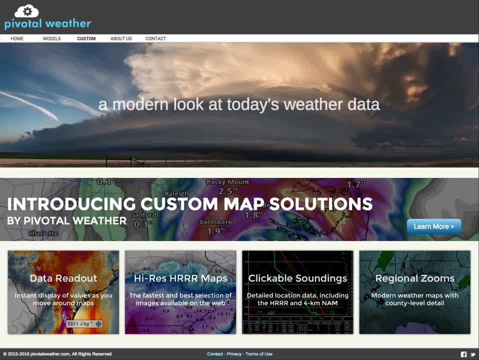 of parameters that we use to forecast the weather. just really briefly, But I'm just going to walk you through this website so that you can use it, so that you can follow along my forecast breakdown videos. You can use this along with me. So that's going to be short and 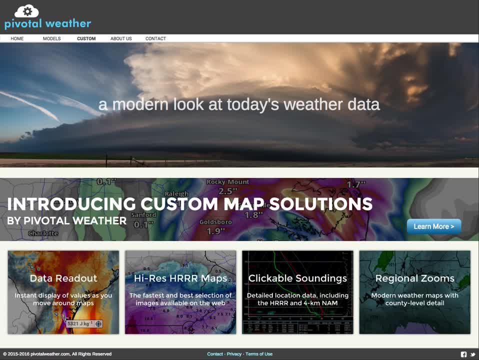 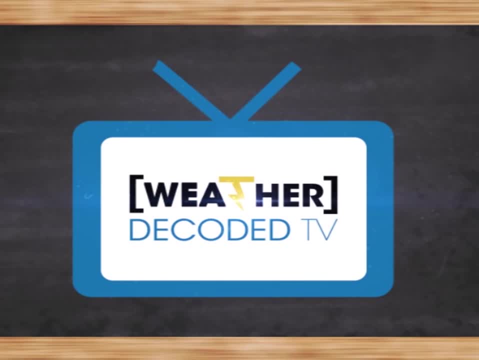 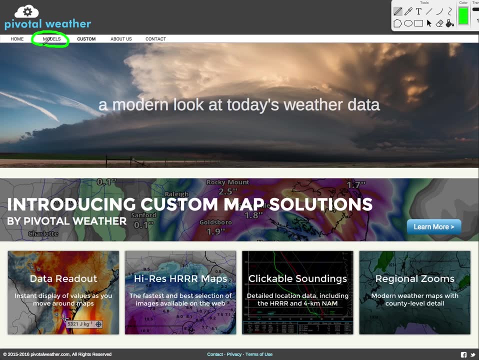 sweet, but you should get most of what you need to know here within this video, So let's crack into it Now. most of what you're going to need on this website is going to be in this models page, right here. In fact, pretty much everything is. I'm going to click on models because that's where 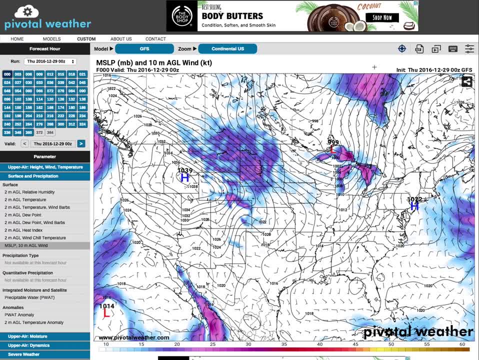 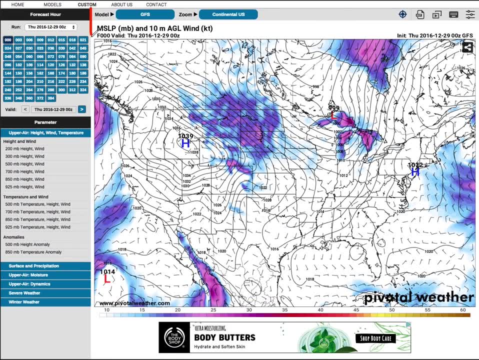 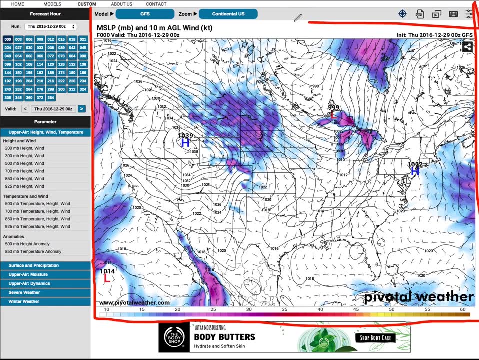 we're going to be for most of this tutorial here, So this is our default page when we click on models, And I'm just going to break down the structure here real quick. okay, So this stuff right in the middle, Well, this image right here in the middle is obviously our map. Okay, Right. 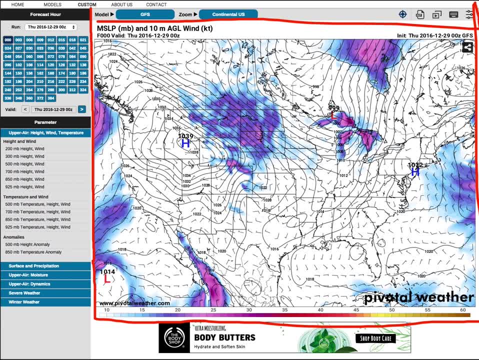 there, how to drop a box around there for whatever reason. But I'm going to. I'll break down what's on this map here. Below usually is where the scale is found of whatever parameter you're using. So in this case it's wind, So you'll see your wind speeds down here and they'll be. 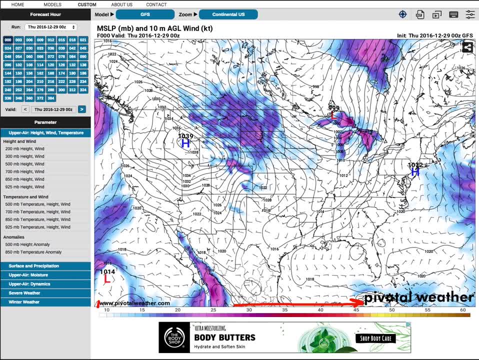 color coded, okay, Usually the smallest over here, the highest over here, okay, And I'm going to actually Up here- will be your label of your parameter that you're looking at. Okay, so we're looking at pressure, the surface pressure and the wind up here. okay, 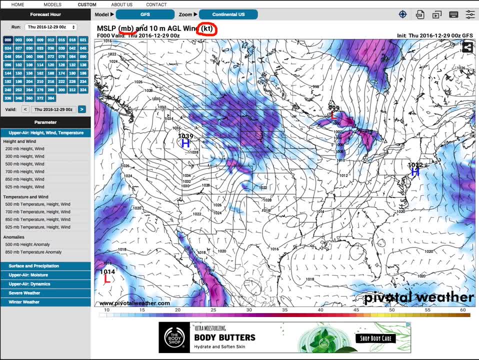 The KT is the unit of measure: knots, MB, millibars. Now, as we get over here, this is when the model was made or when it was ran. okay, When they run it. you know the good old supercomputers. 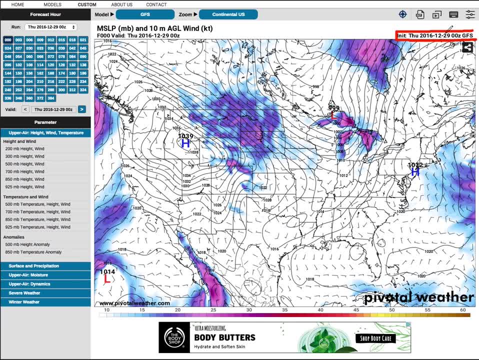 when they run it. It was ran on Thursday, December 29th 2016, at zero Z. Now, zero Z is a time, a measure of time. like you know, 5 pm Eastern is, for instance. 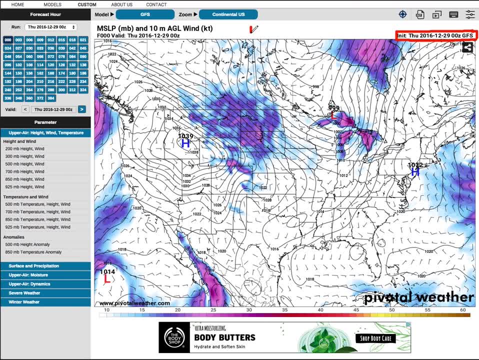 Zero Z is a measure of time and it's similar. it's actually UTC, universal time. okay, It goes from zero to 24.. And so if you wanna know what zero Z actually corresponds to, like in the central US, it corresponds to 6 or 7 pm. 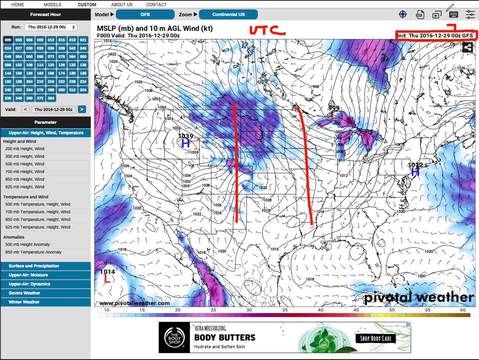 depending on if it's standard time or central daylight time. If you wanna know those conversions, I actually have made a tutorial on that. You can click on the link in the description below and I give you a table. You can take a picture of it or whatever. 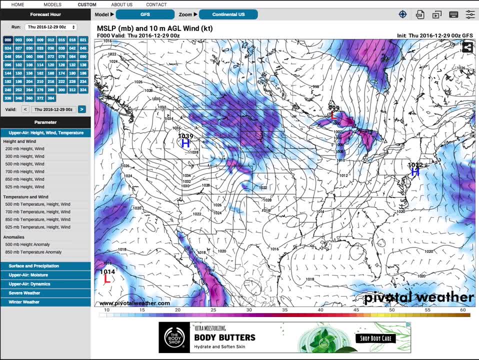 and you can kinda use that as your cheat sheet. So that's the time. Now. the model that we're looking at is the GFS. This is the computer model we're looking at, okay, And there's plenty of different models. 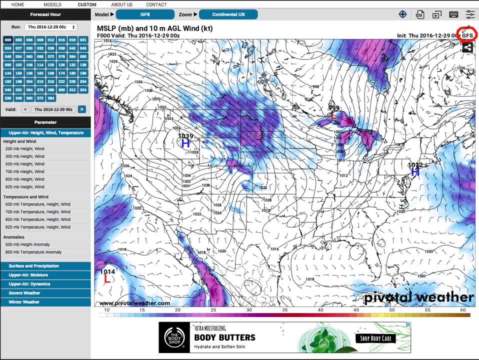 We'll go over that in a second, But what we're looking at is the GFS, the American model. Now over here, this little box right here, F000, F essentially means okay. how far in advance is this? 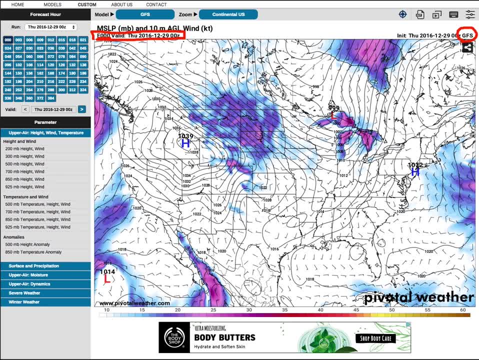 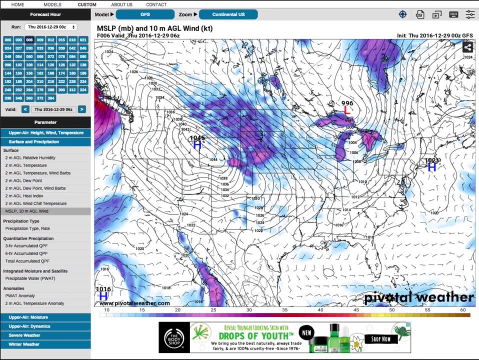 Right now. 00 means that it's current. okay, If we click into the future, maybe like six frames or six hours, you'll see it says F006.. That just means it's six hours into the future And it also says when it's valid for when the forecast. 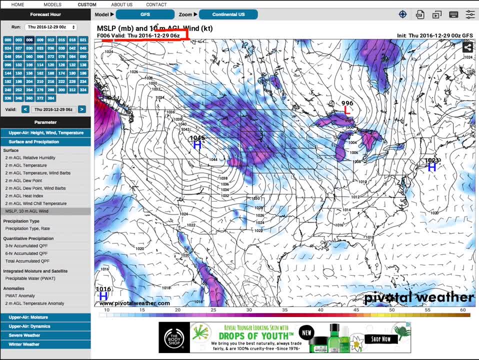 when the model image is what it's forecasting for, And it's forecasting for December 29th, Thursday, 2016,. at six Z, six hours from now. okay, This is when the model was initialized. the current time. 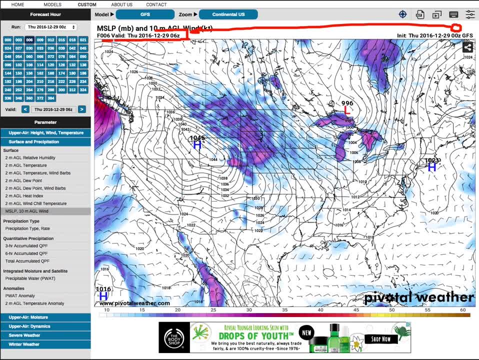 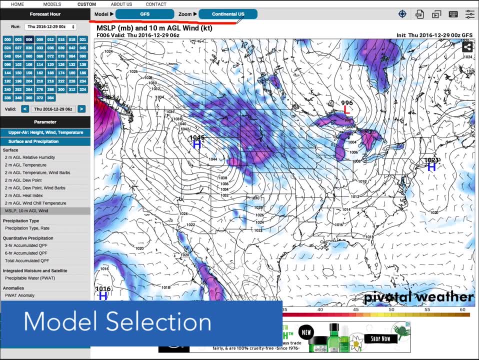 This is the forecast, So it's six hours in advance. it's six Z, okay. So that's kinda the basics of the map. All righty, now this little section we're gonna talk about. to talk about this section right here. okay, this is where we can find our models and our regions. 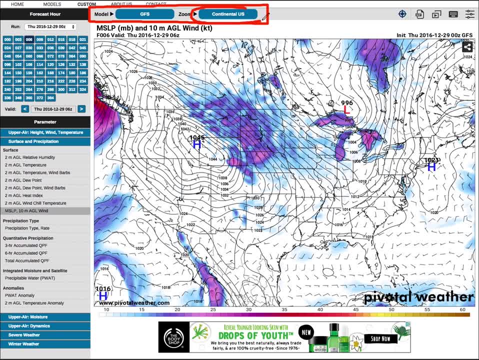 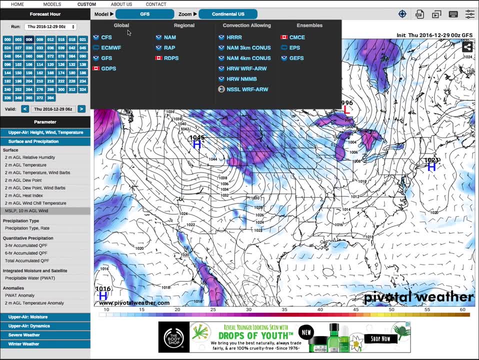 okay, the regions that we want to look at. so if we want to zoom in, zoom out, we'll click on that button. if we want to look at a different model, we'll click on this button. okay, so i'm going to click on this. and there are different types of models. okay, global models essentially cover the 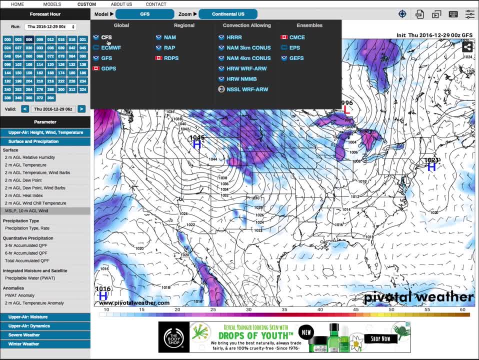 entire globe. okay, and that's the cfs climate forecasting system, your european computer model, which is the ecmwf, the gfs, which is the american model, and the gtps, which is the canadian model. so you can look at all of those, and these global models are more broad. they're good at examining. 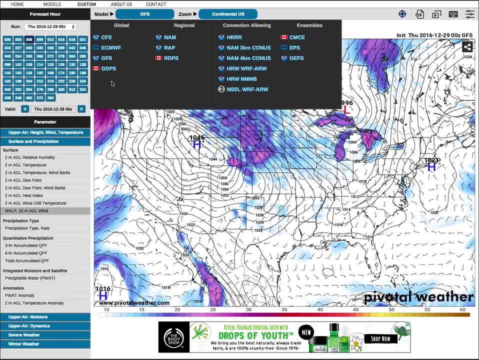 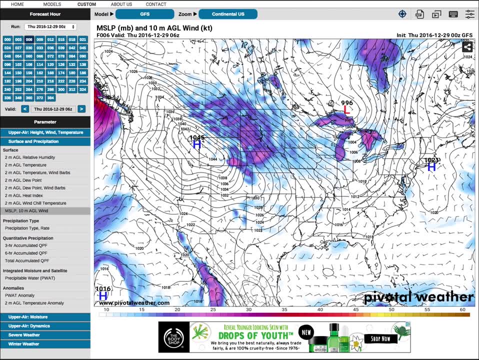 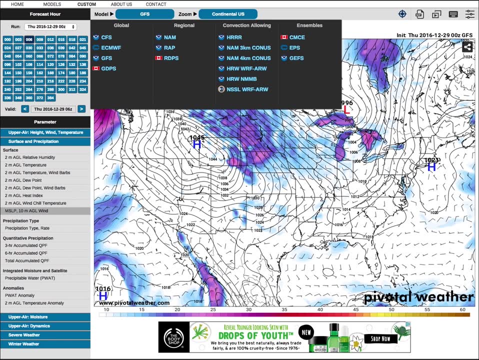 weather patterns and they go well into the future. okay, like two weeks, as much as two weeks into the future. these regional models right here- oops, we'll go back to that- the regional models, those examine kind of a little. they're better at examining shorter term, more detailed weather events. that's the nam, the rap and the rd dps. okay, that's the. 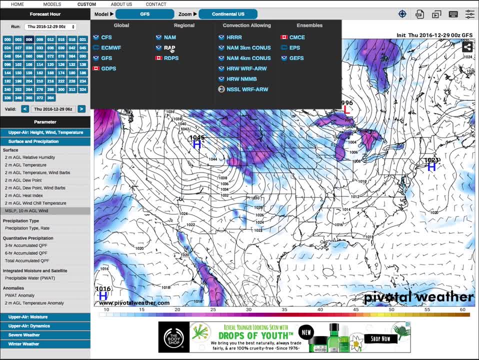 canadian version. the rap is actually the highest resolution of all of them and you can get really fine details like where storms are going to develop. uh, you know, it shows tornado potential. some very, very fine detail. okay, that's what these regional models are, these convection allowing. 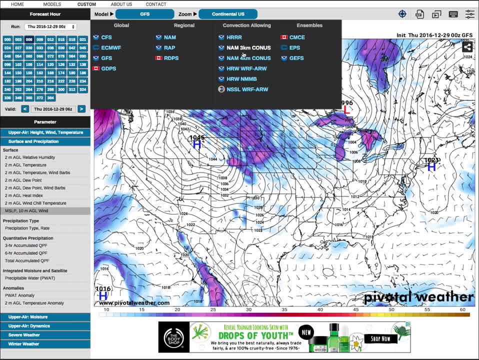 models. actually, a lot of these are the nam- okay, the nam 3, cam, 4, cam, hrw, and so you got all these different versions of the nam and the wrf here and the hrr, which is the high resolution rap we were talking about. now this gets extremely detailed at the mesoscale level, which is essentially the thunderstorm level. 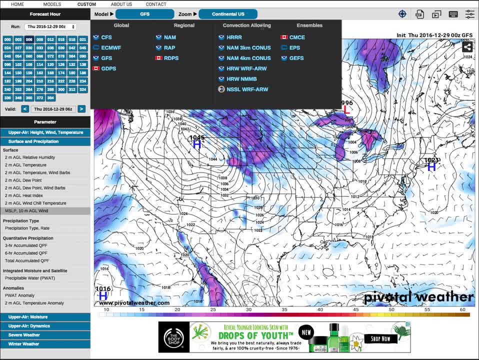 okay, so you can really a convection allowing essentially means it'll show you simulated reflectivity, so like radar, into the future, so you can really see the future and then you can kind of see the what the radar is going to look into the future, if you ever seen those. 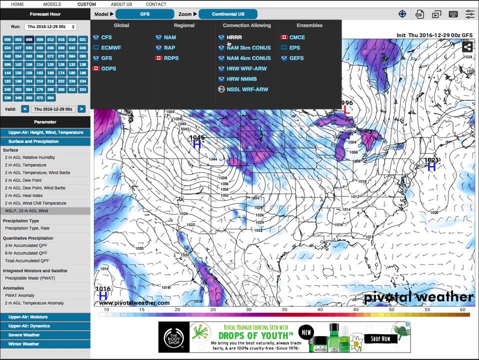 apps. it's likely one of these models. here there's several different kinds, the hrr and the nam 4k, and, being the most popular ones, you can examine lightning, all that type of stuff. so let me just kind of show you real fast like what i mean: the composite reflectivity. uh, that's what this is. 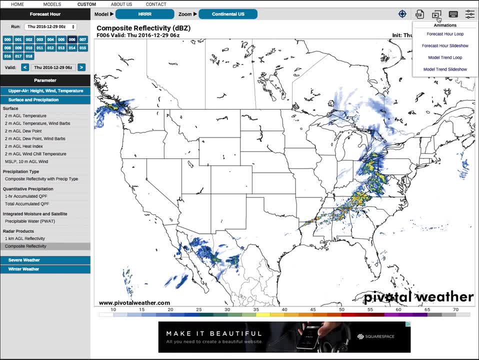 and you can see the radar in advance here, six hours in advance, and you know you can go into, go into the future. we'll go over that in a second, but you can kind of see the radar. what you see is: well, you can see how highly refreshed it looks. it's really great overview. uh, look at that. 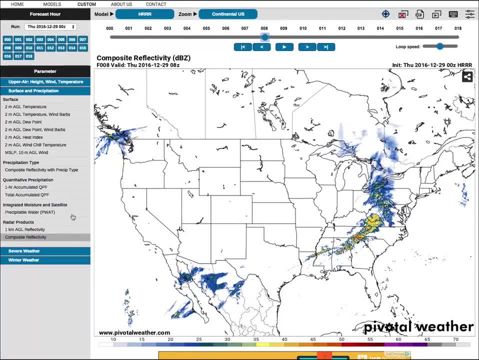 so you can assign it to each other as well. you can say: look at your radar, you can kind of use it and gently dusk. you know that we got it when some things are off, that it's fine, we'll kind of use it. You can kind of see the radar and there's all these different types of stuff that examines. 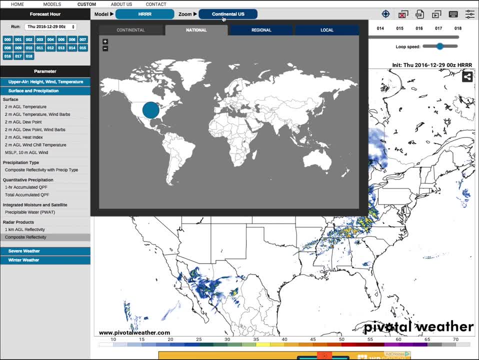 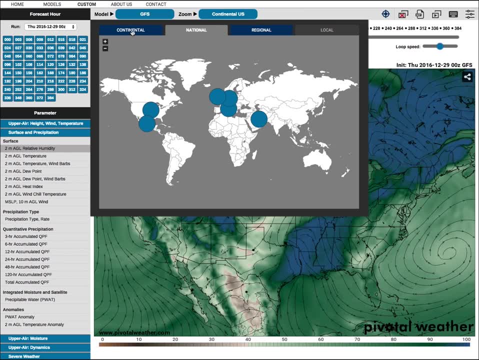 a high level of detail. Now, this thing right here, we'll go back. we're going to go to the GFS. click on the global model. This thing right here shows you all of the regions. With the global models you can do different continents. 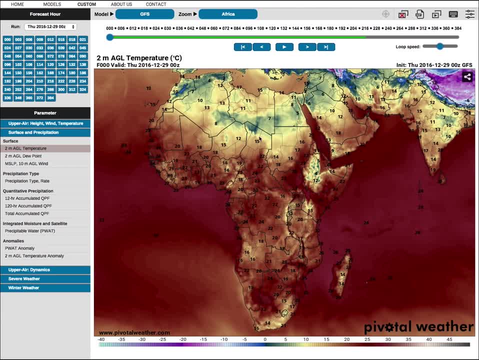 So you can go over to Africa and say, hey, what up, What up, And you can look at all of Africa's weather. It's pretty cool. You can watch hurricanes and all that stuff go off Africa and make their way onto the east coast or whatever. 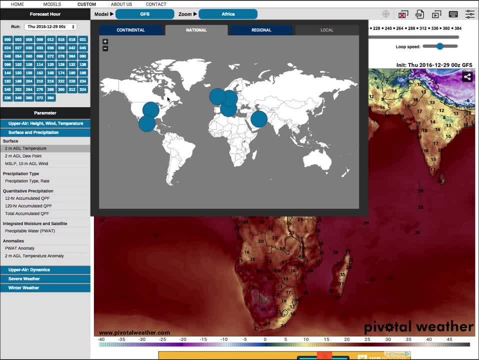 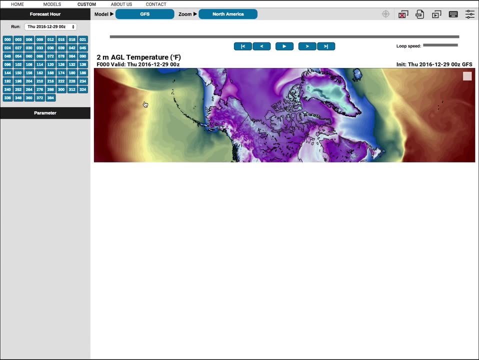 South America, Australia, all of that, So you can look at national views: Mexico, North America or the United States, parts of Europe. That's going to be good for weather patterns And this is going to be the continental views, or, like North America, 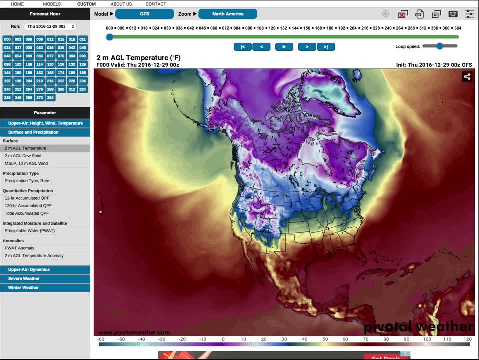 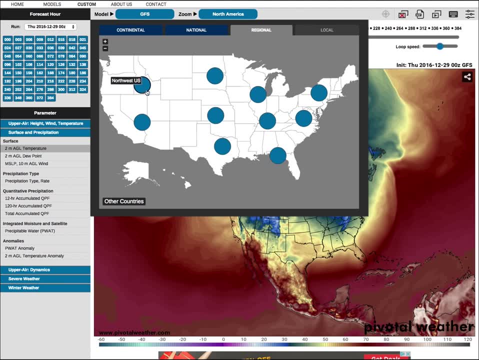 That's very good for long range weather forecasting. You've got really broad patterns. Then you've got regional. It's only offered for the United States here, But you can go like the Northwest, Southwest, Southern United States, Southeast. We'll click on the Central US and I'll show you what that looks like. 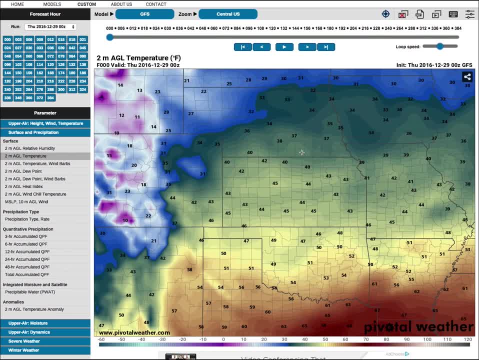 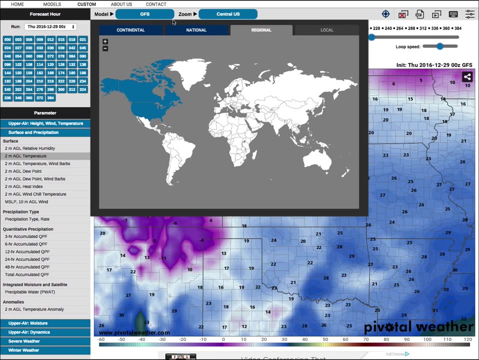 So it's kind of zoomed in and you can see much finer detail. This is good for examining winter storms, severe weather setups or just your highs and lows for the day, whatever. So that's regional And then local. Okay, Local is actually something you're only going to get with the – I believe the – we'll. 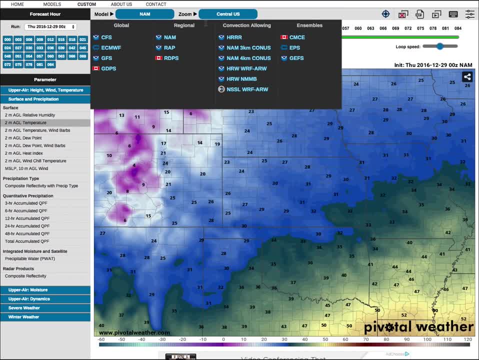 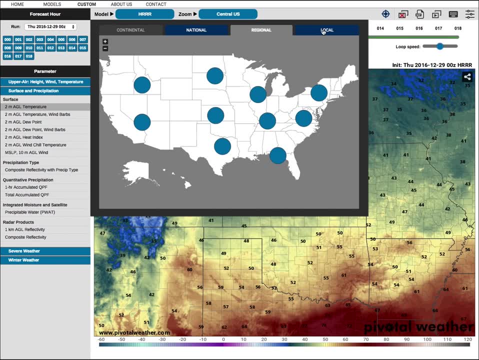 check regional. Let's see if they have it for that. Now, you're only going to get that for the convection allowing models, which is the really tight zoomed in models such as the HRRR. We'll go local and we can click on Oklahoma. 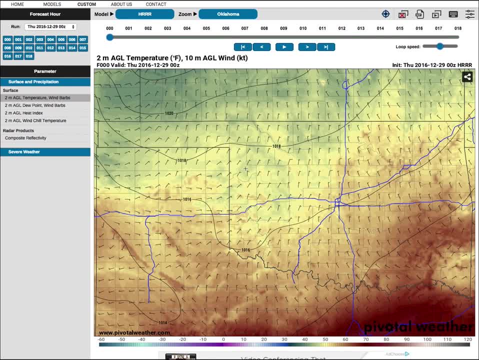 There's actually more that they offer. depending on where the storm is, It'll move around the buttons. You can see you can really zoom in here. You can get down to like – Where things are near interstates and stuff, There's more wind barbs. 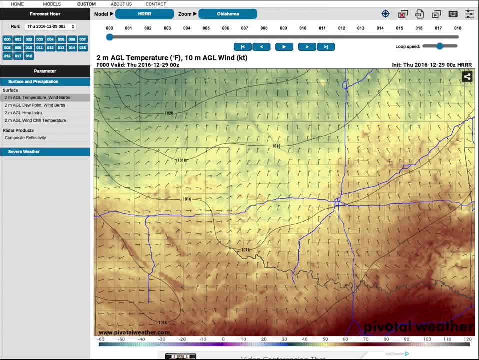 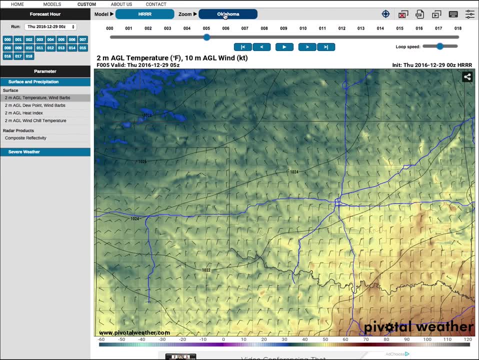 It's finer detail, So that's kind of cool like that And you can really see fine detail. It's good for severe weather in particular, or like forecasting snow bands and stuff like that. So one thing I actually forgot is this thing: right here ensembles. 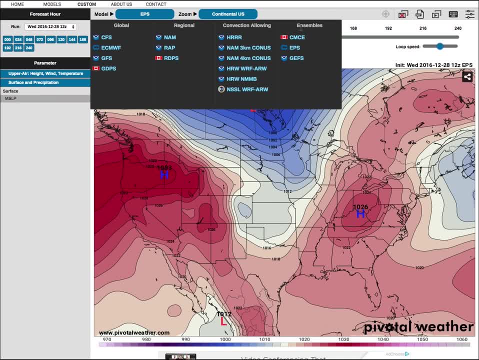 We can click on EPS here. Ensembles are essentially a bunch of model runs stacked together of the same model. So like the European will run a bunch of different variations of the same run, Like they'll change the temperature up slightly and then they'll stack them all together. 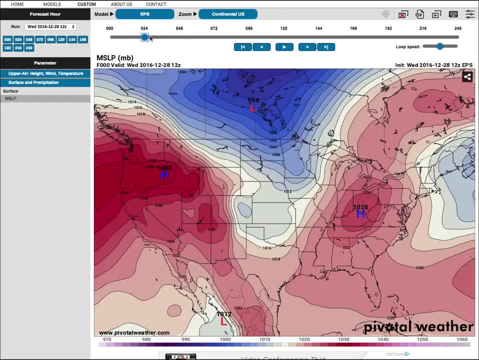 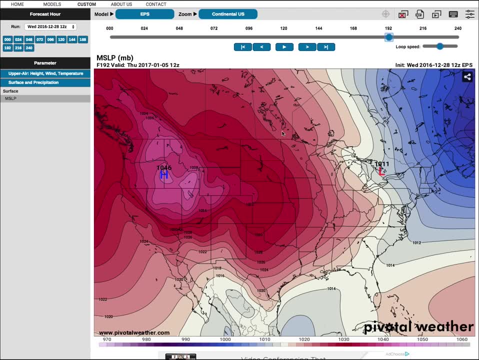 And so it's just kind of a blended composite, And so these are kind of – they're not as detailed, but they show confidence. So there's a lot of confidence, There'll be warm air here. but it's not as detailed. It just kind of is more of a confidence model. 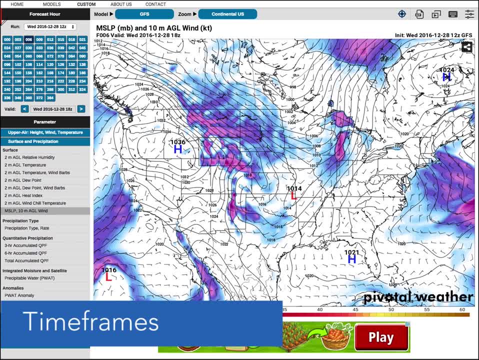 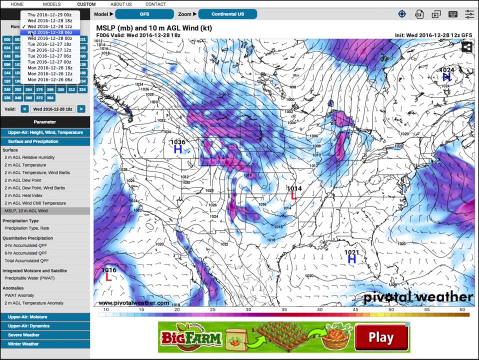 All righty, next, What is up next? Let's talk about this box right here, this little area right here, okay, And so this section shows your forecasting hours and the different model runs Right here. this is where you're going to find your different model runs, okay. 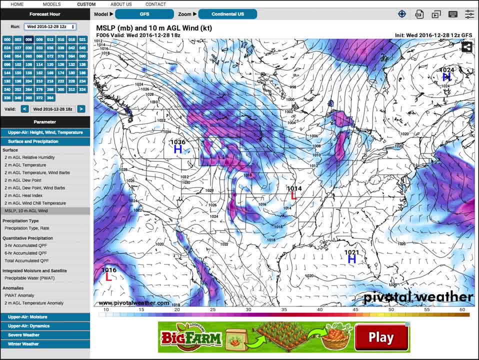 And model runs are essentially – well, you have different models, and some are ran four times a day, four times. Some are ran every hour, which is 24 times, like the high-resolution models, And some models are only run 24 times a day. 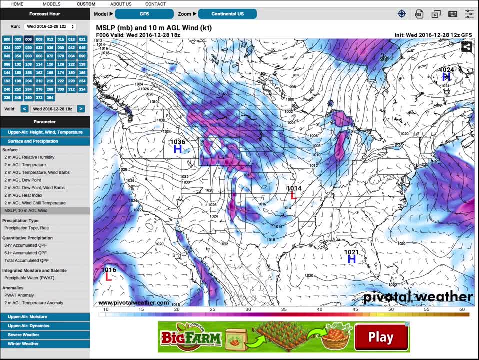 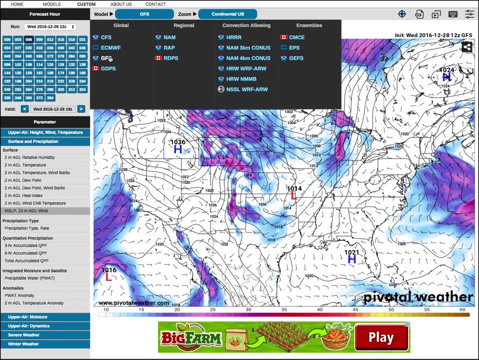 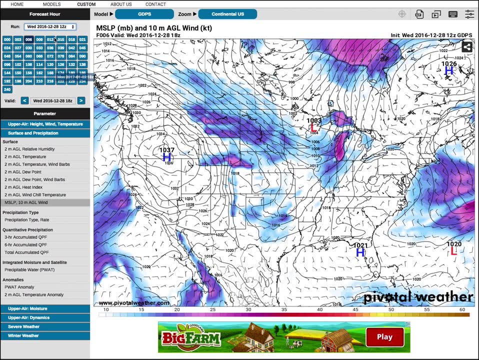 Okay, Some models are only ran like two times a day, usually the international, like the Canadian and the European. Actually, I think the Canadian might be ran four times. No, it's actually two times here. So that's going to be your model runs. 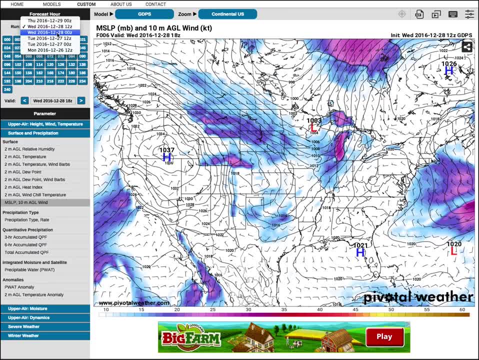 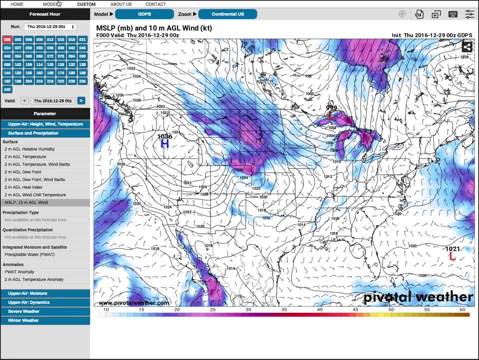 And you can go back in time. So if you want to see an old run from six hours ago, you just go back one tick, or even maybe a couple of days ago. you can go back that far, okay, And so you can kind of see how the model has been behaving that way. 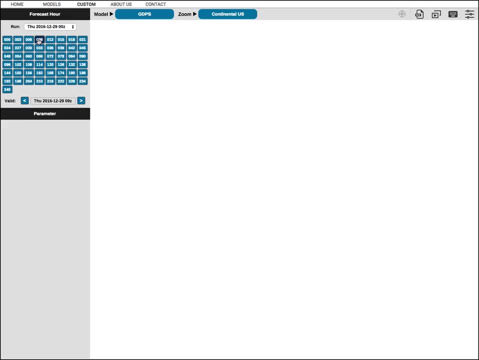 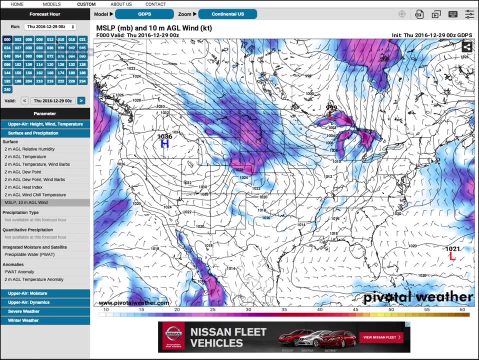 So this thing right here down here is your hours, So you can go farther in advance. It's like nine hours in advance. This is currently the 000, 15-hour advance. hey, where is that That's going to be right there? 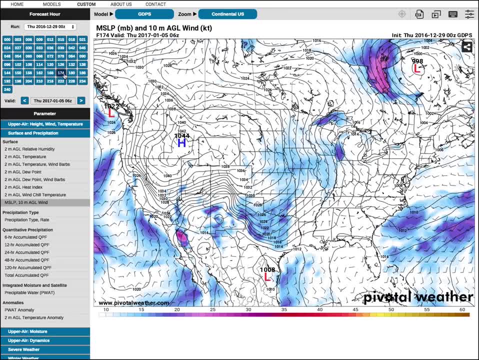 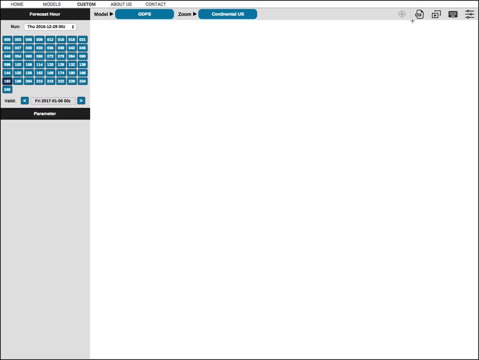 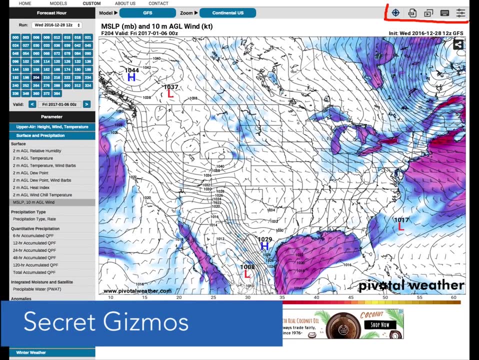 If you want 174 hours in advance, you click that right there, okay, And then you can also just click the buttons down here as well. So, that being said, that is that little box right there. Next up is all these little secret gizmos. 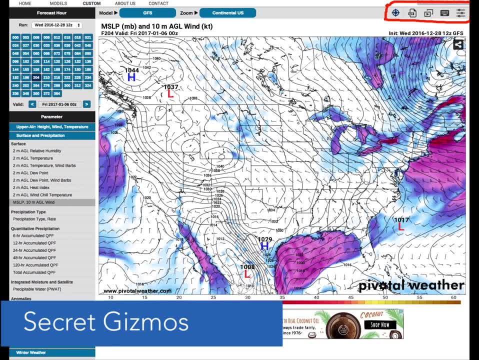 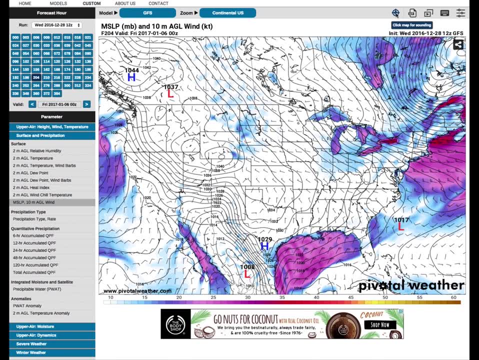 In the corner here. okay, I'm going to talk about those now We'll talk about. let's talk about this thing first. This little thing is a little target And when you click on the map, watch what happens: boom. 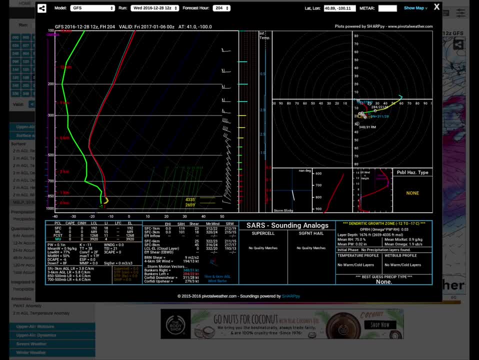 This is called a sounding And this is a Sharpie. This is actually what Sharpie is, but that's for another day. But these are soundings. They're vertical profiles of that point I chose on the map, So I think I picked the middle one. 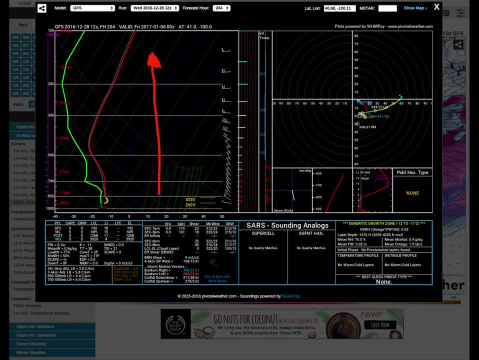 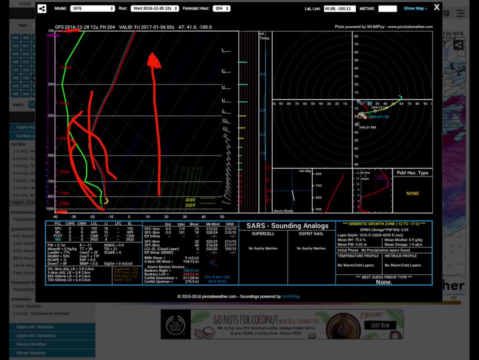 The middle of the United States. So it shows what the atmosphere looks like in the vertical, from the surface up to the mid-levels. It shows temperature dew point. dew point temperature, wind speeds over here, all sorts of little variables. Again, this is a tutorial for another day. 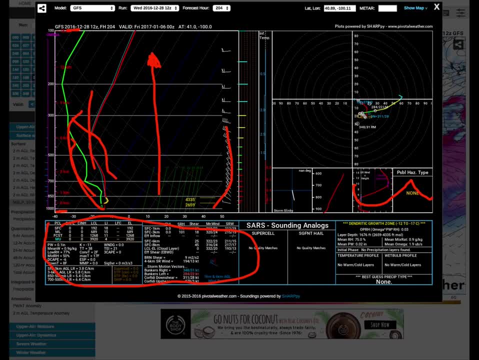 I mean, you could probably spend hours on this And then your possible hazard type out here like tornado, snow sleet, whatever. This is a hodograph. It shows the winds and the atmosphere, And this is for another day. 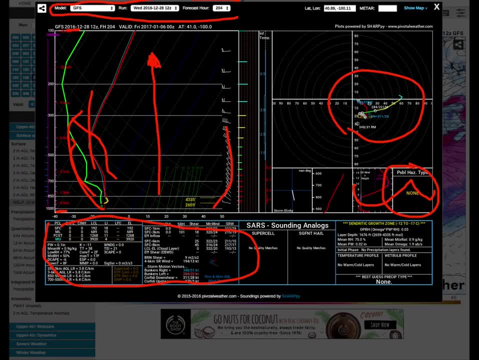 But you have all of your kind of your same stuff up here. You can change models, You can change the run, the forecast hour up here, This little button here you can share it. Latitude and longitude. So if you want to choose a different location based off latitude and longitude, just type. 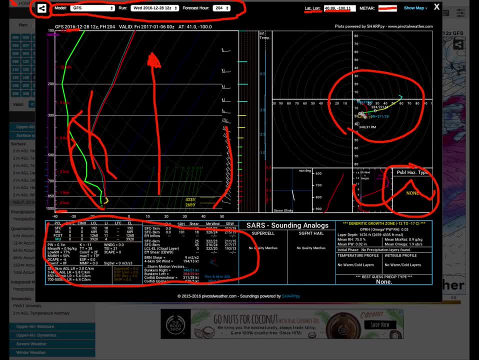 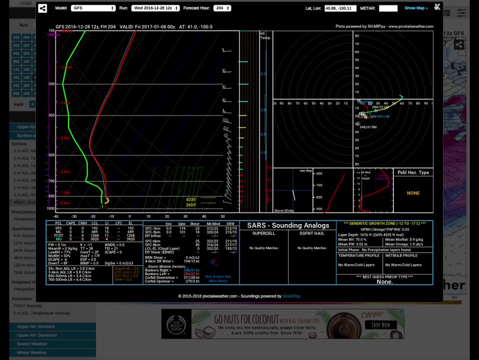 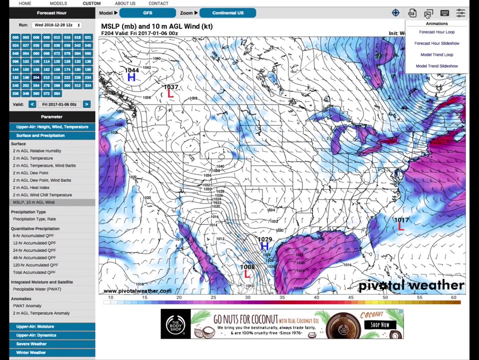 it in right up there. Then this is a METAR. You get little codes for that, But again, this is for another day, But anyway that's a sounding. So those have a lot of information. They're very useful. Let's see this thing right here, this little play button right here you can kind of view. 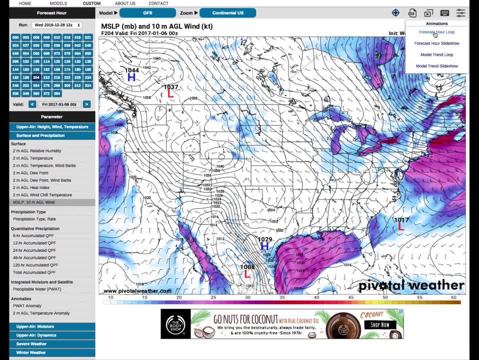 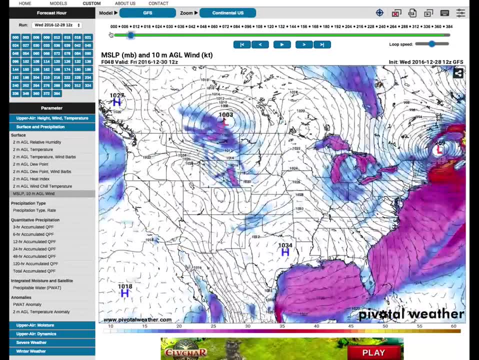 different views of this model. So you can click on forecast hour loop right here. This will show an animation. You can drag this thing. This will show animation into the future. You can click the play button. It will just automatically play it. 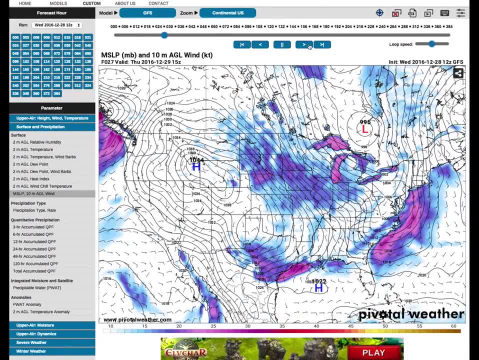 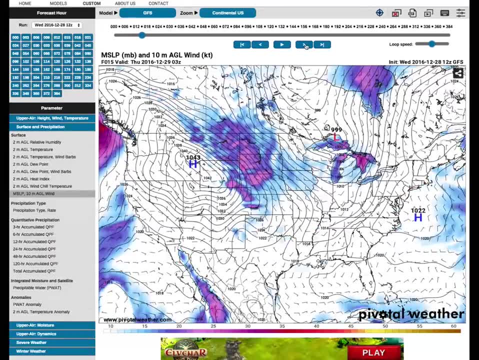 This is to speed it up, slow it down when it plays. This is to go to the end. This is to go back to the beginning. I think actually, these are just to go one at a time. So if you just want to go, click it one at a time. 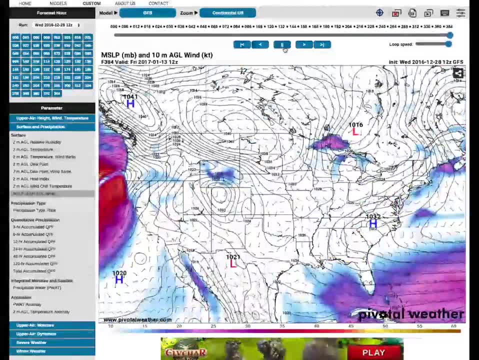 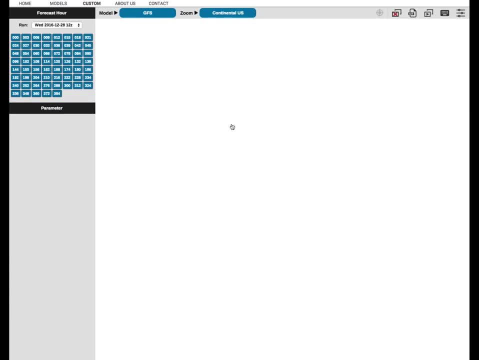 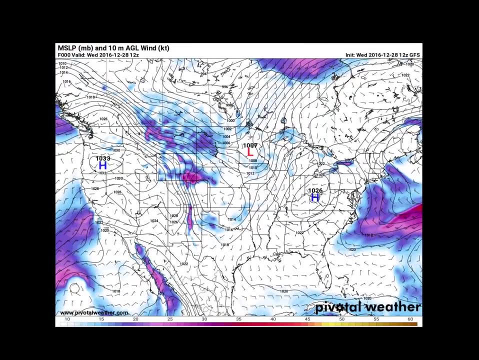 This is the loop speed right here. if you want it to play faster, That's ridiculously fast. there We also can click on forecast hour slide show, And so you can just kind of click on a button or a thumbnail And you can use your arrow keys on your keyboard to fast forward and go back. 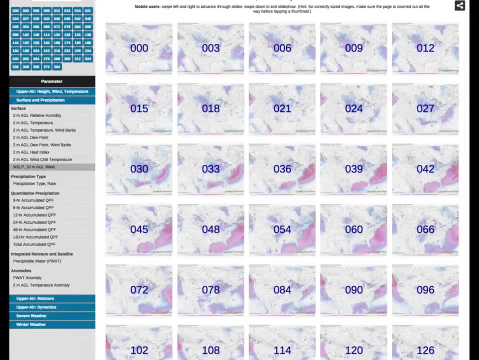 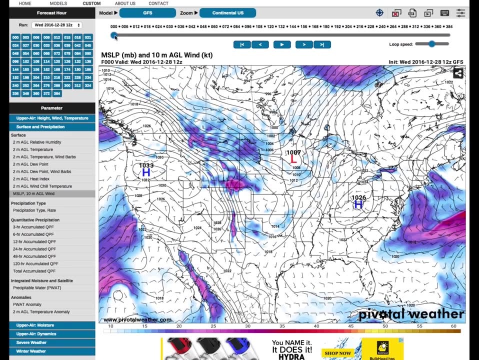 I think that's a lot of fun too, just clicking your arrows on your keyboard, So you can do that with that, And I think there's a way you can do that on the loop as well. If you click this blue button right here, make sure it's selected. you can now click. 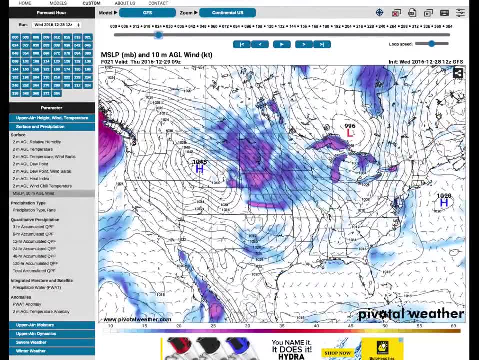 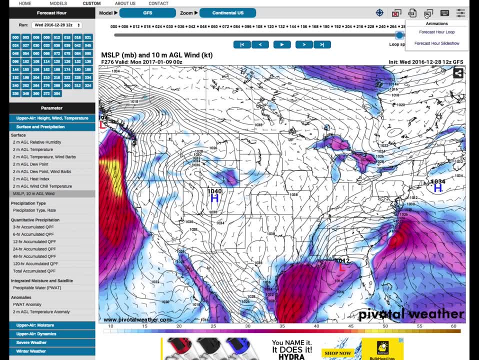 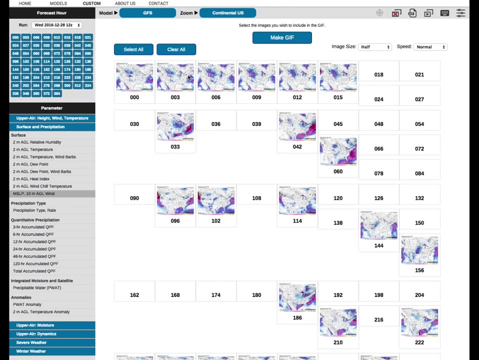 or you can now press the buttons on your keyboard to go back and forth. I find that's very convenient. I like doing that the most. So, that being said, that's how you animate. Hey, If you want to export Something as a GIF, like as a little animation, if you want to share it on Facebook or whatever, 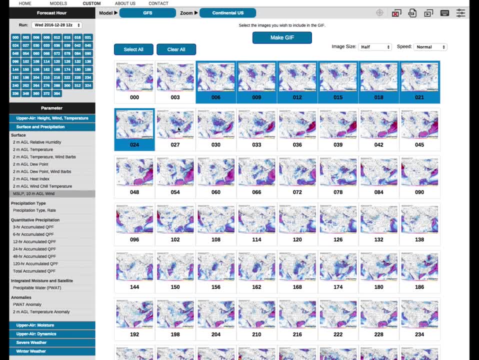 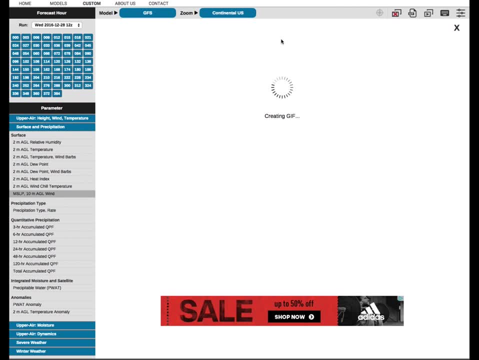 You can click whatever button or whatever images you want in your GIF. You can choose your size, the speed, how fast it animates and you can make a GIF. It'll doctor up a GIF for you And look at that. It's animating and stuff. 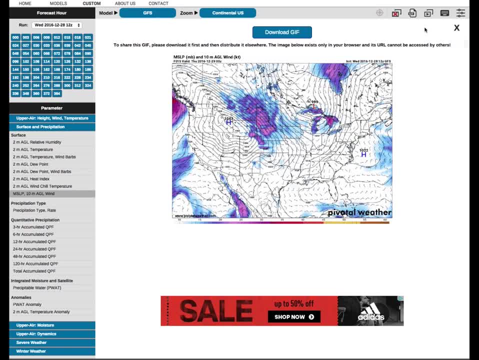 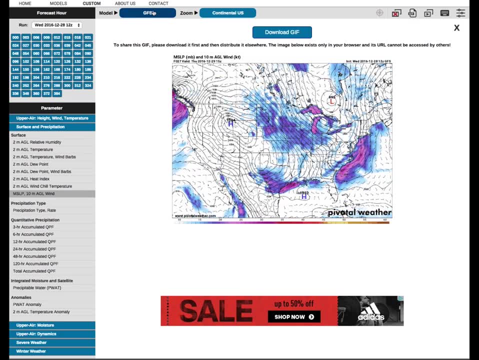 And so you can actually save this image onto your desktop, share it, do whatever you want. So that's how you do that. Now, this thing right here: these are codes that you can use like little keyboard shortcuts that you can use. 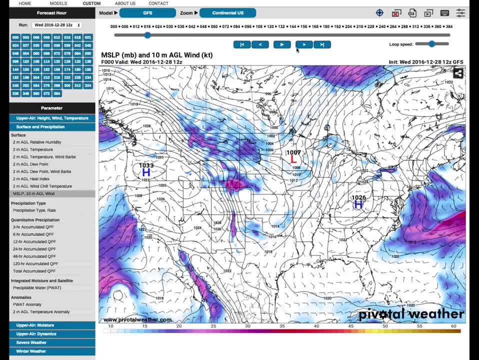 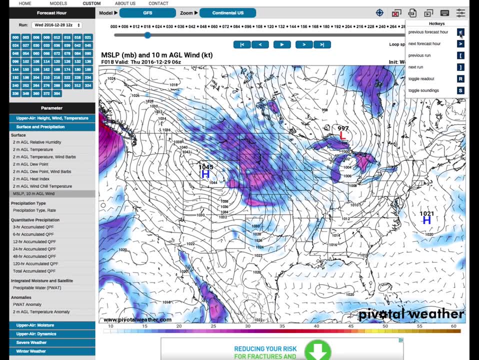 We have to exit the GIF here somehow. Let's go back to forecast our loop. These things right here are keyboard shortcuts. So again, that's the previous button on your keyboard, That's your forward button, If you want to go to a previous model run. 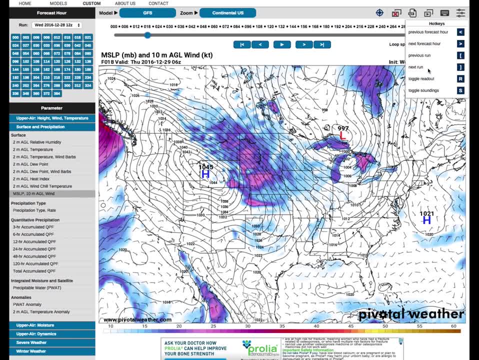 Hit the brackets. okay, right there, the next run. The toggle readout button- I'll get into that in a second. The toggle soundings: Well, that soundings button we just went over when you click on the map and you can click. 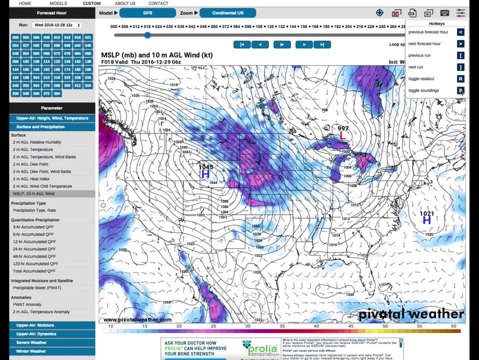 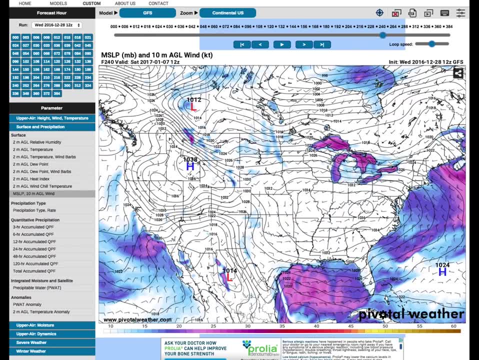 a sounding. it comes up like that: If you don't want that, you can hit the key S. Just hit S and when you click it doesn't pop up. Sometimes that can be annoying. Sometimes you'll accidentally click and a sounding will pop up. 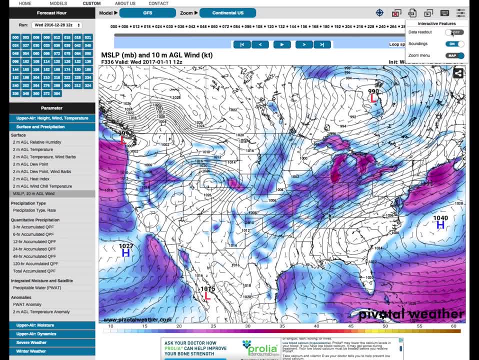 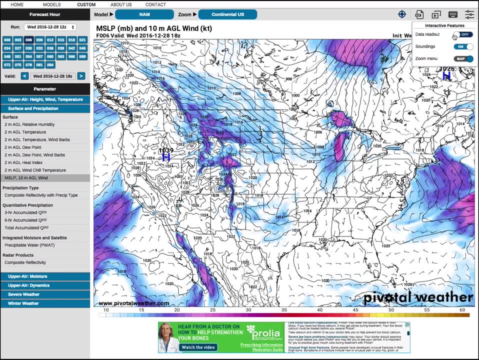 So if you want to turn that off, you can hit S Okay, Or you can go over here and you can click off on the soundings right here. That'll work. There you go. Okay, There's this really cool feature. 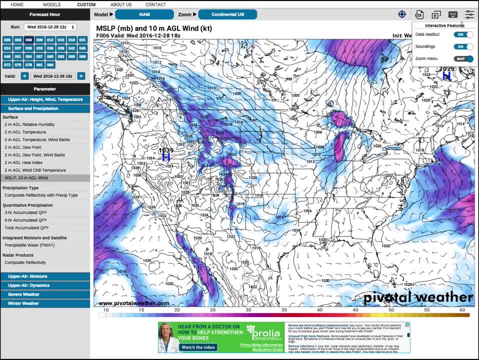 It's called data readout. Data readout- You can click it on and off, Or you can go to your keyboard and click R. You can hit R, It'll turn on and it'll turn off. Essentially what that is. it shows you the value. 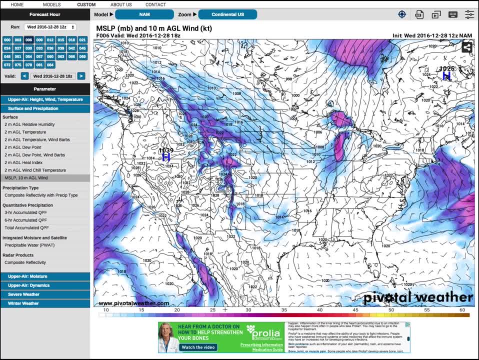 See that little box that popped up. This is examining wind speeds. You can see, right here in southern Montana the winds are 19 knots. Wherever you go it'll change and stuff. That's kind of cool if you want specific detailed variables there. 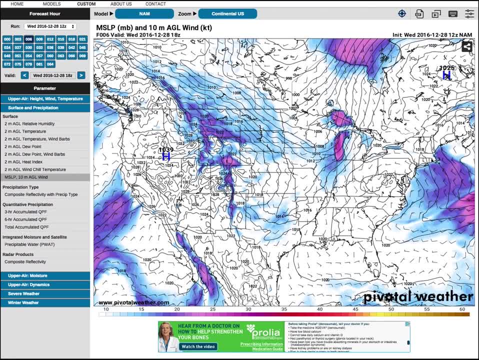 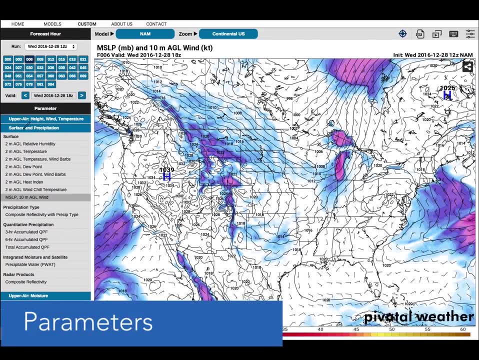 That's kind of cool as well. That's all those gizmos over there. This is a share button right here. Forgot that You can share on Facebook or Twitter. There's that All right On to our final section here. 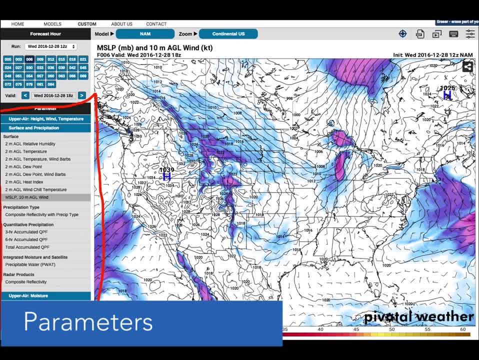 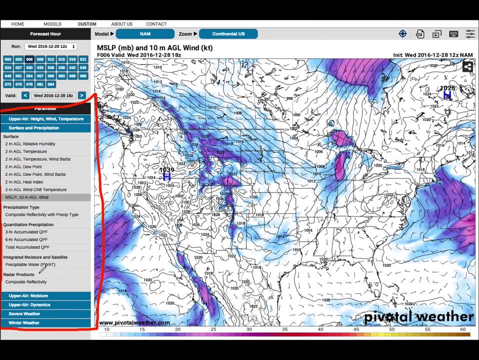 This box right here. This is where the fun stuff comes in. These, These buttons in here are all our different parameters: Our temperatures, our snowfall accumulations, tornado potential. You're going to find all of that stuff in here. There is a lot of that stuff. 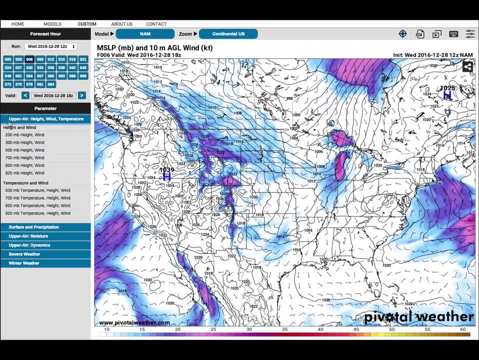 Each of these are divided into the little different sections. The first one is upper air. That's examining the higher levels of the atmosphere, like the jet stream, But it can also go down to near the surface. That's just Especially in this right. here you're examining wind, heights, temperatures. 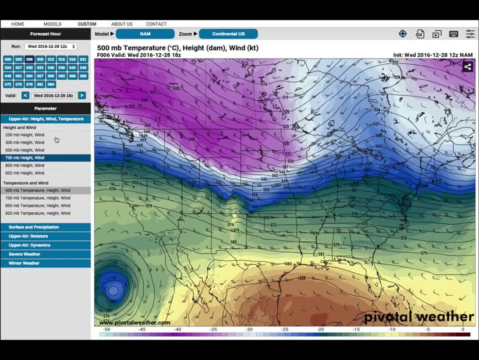 These are height lines. Now I can make a tutorial on all of these, but again that would take hours and stuff. That's probably for another day. I'm not going to go over each of these, but I'll just briefly talk about what you can. 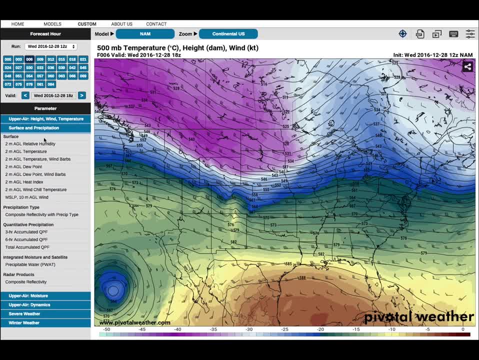 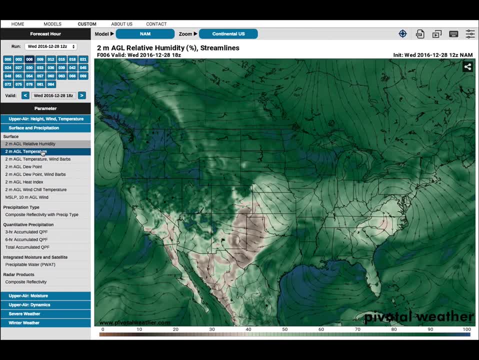 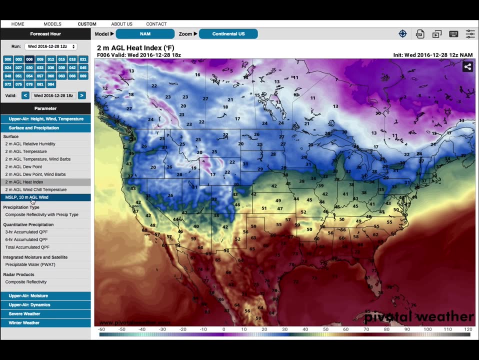 find in each second section: Surface and precipitation. This is where we're going to find humidity, surface kind of the stuff we experience ourselves at the surface: Temperature, dew points, humidity, heat index. you can find the wind, chill, the pressure. 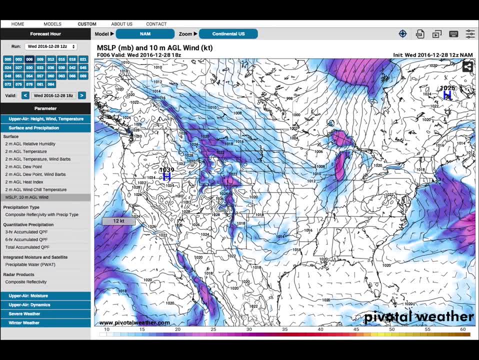 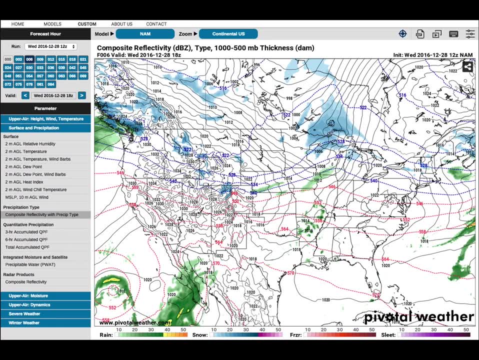 and the wind, the wind direction, the wind speed. This thing right here is called composite reflectivity and that is radar into the future. All the models have that. You can see that. you can look at snow, freezing rain, sleet rain. 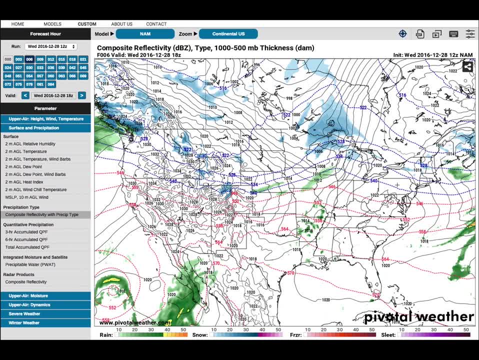 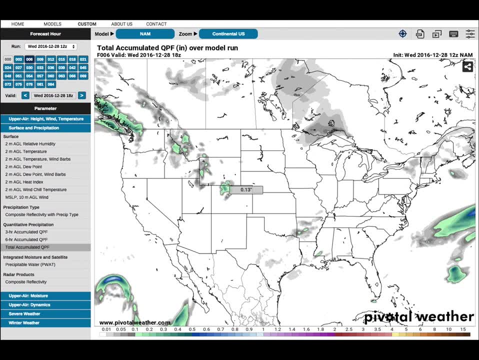 That one's really fun Thickness. These are these dashed lines. That's the average temperature in the atmosphere. You can look at quantitative precipitation. That's essentially what that is is how much liquid precipitation falls. You can see up here: there's 0.6 inches. 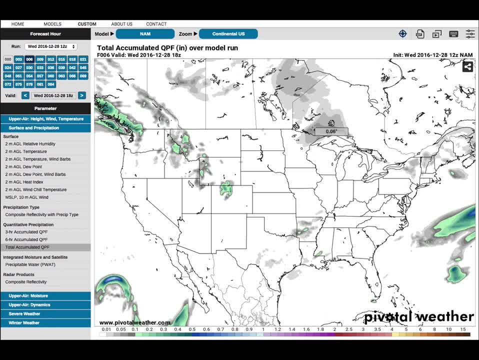 That's not 0.6 inches of snow. well, it's 0.06.. It's 0.06 inches of liquid, and so you can actually translate that to snow, which is probably like 0.6 inches of snow. 10 to 1 ratio. 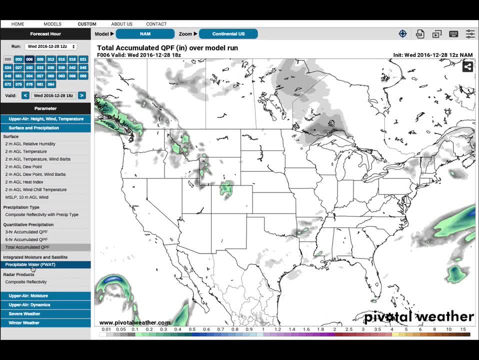 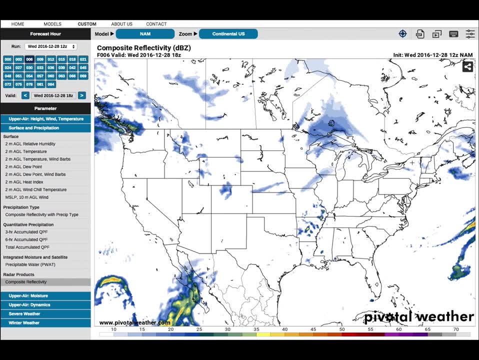 It's just so simple. It's showing how much liquid there is. Precipital water measures moisture depth in the atmosphere, how deep the moisture is. Here's another composite reflectivity that doesn't show precipitation type. This section right here is upper air and it's examining the moisture. so that's going. 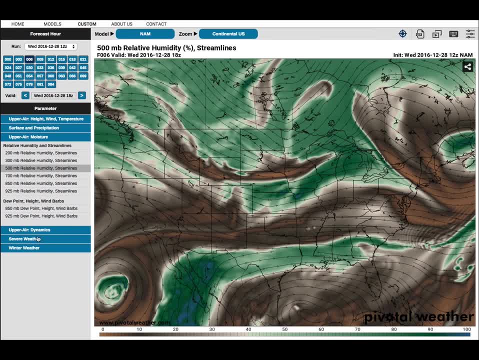 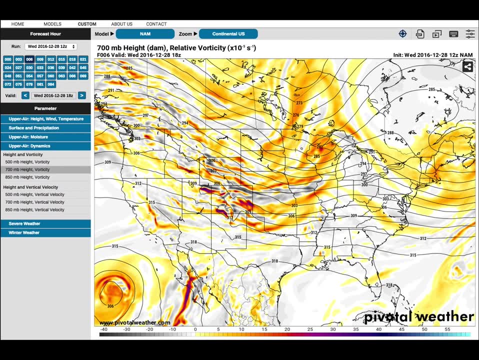 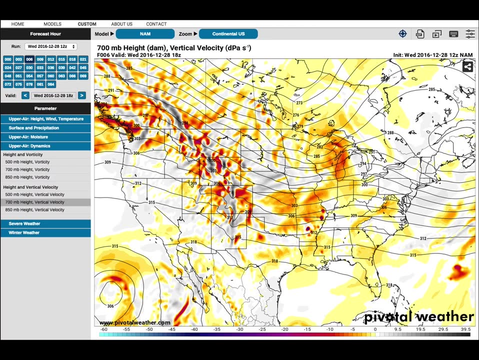 to examine your humidity and dew points in the upper levels of the atmosphere, Upper air dynamic section. that kind of shows how much lift is in the jet stream, the vorticity, the air flow, The speed, the spin, the vertical velocity, how fast things are moving upwards or whatever. 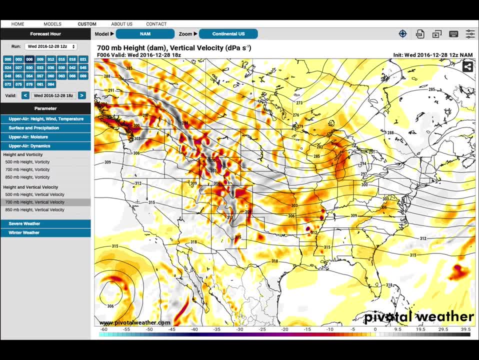 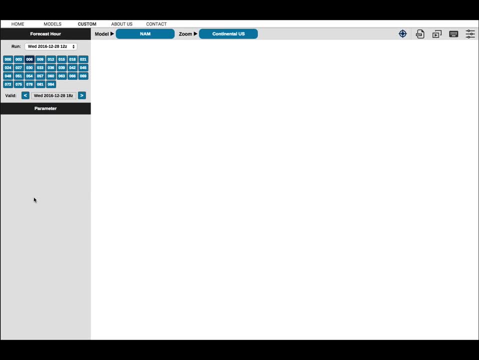 That's going to be there. That's good for examining storm systems like giant broad scale synoptic storm systems and even some rotation and stuff like that Severe weather that's going to be predominantly in the spring season and summer season. You can measure your instability: your wind shear, your cloud base height. 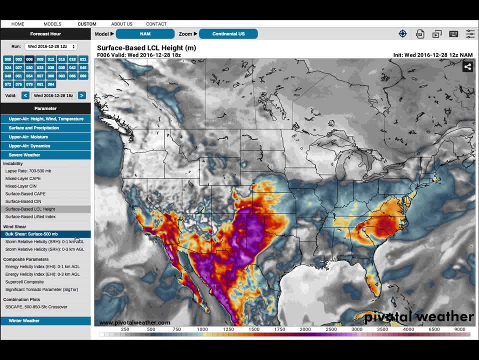 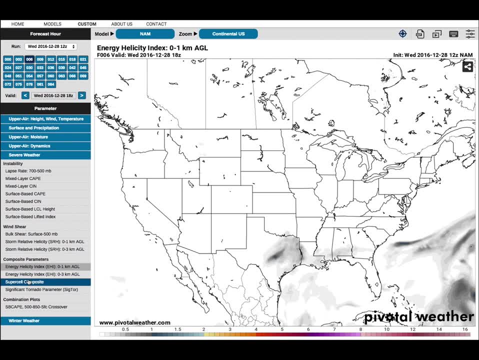 How fast the temperatures fall with height, your wind shear, how much spin is in the atmosphere for tornadoes. You have some indices here that show you the tornado potential: Supercell composite which shows the potential for supercells You may like down in Texas it's a little bit elevated there. 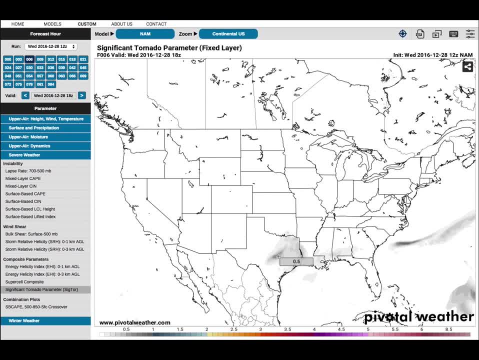 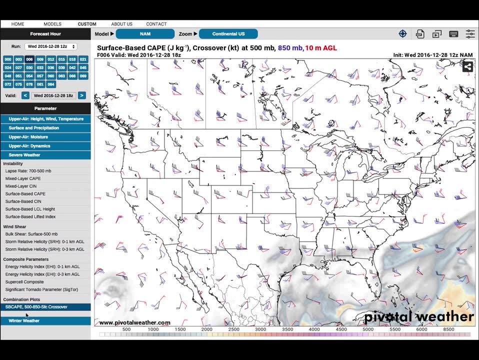 Significant tornado parameter shows the potential for tornadoes. Whenever it's above one, usually there's a chance at a tornado. It's not always accurate, but that's that. This crossover is instability and wind shear on top of each other. Whenever you have something called composite or crossover, it's usually multiple different. 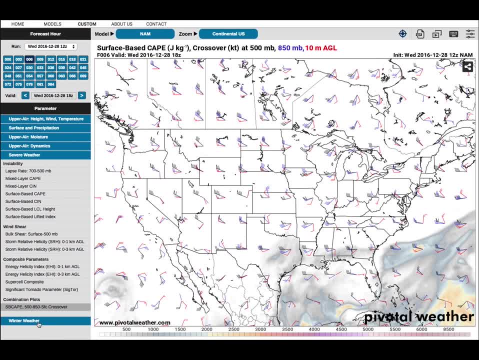 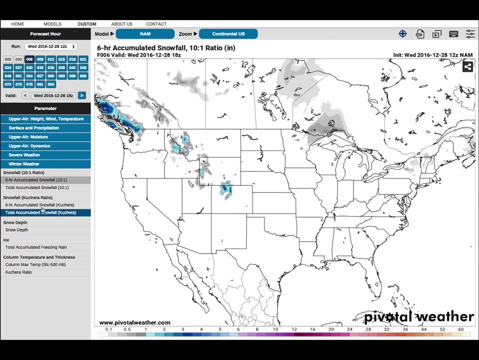 parameters on the same map. This section right here is winter weather. You can go over snowfall accumulations. This is just a different equation that they use to find snowfalls. You can look at both of those. It's a good idea to look at both of them. 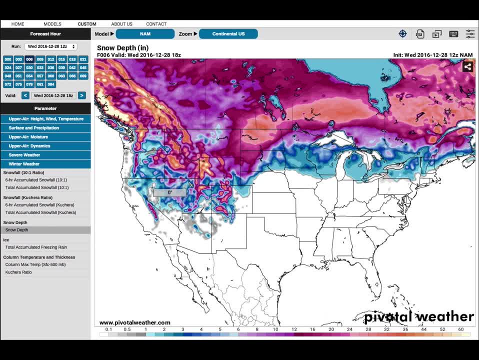 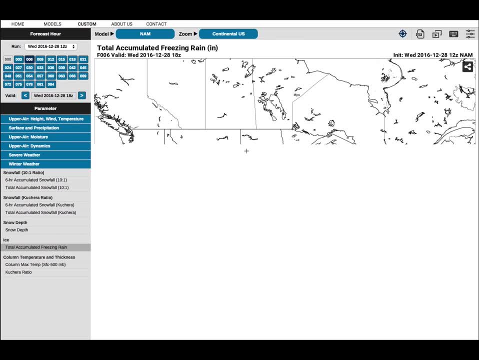 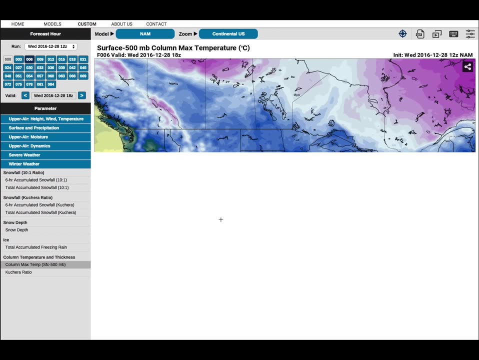 Snow depth shows how much snow is currently on the surface. It's not always accurate, but it's good enough. This shows ice. if there's going to be any ice Right now there's not, but that's freezing rain. Column max temperature. that shows the maximum temperature in the atmosphere from the surface. 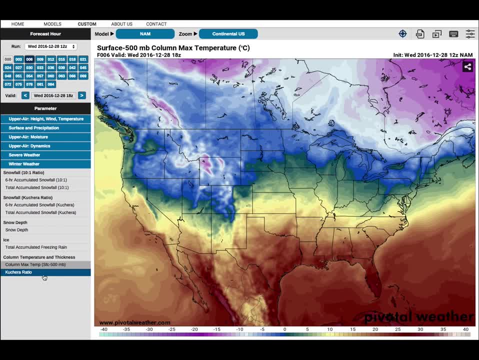 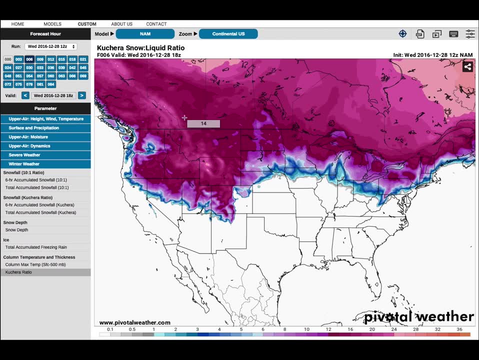 to the jet stream. That's the highest the temperature is. That's good for winter. Then the Couchera ratio: That's good for winter. That's going to be your snow ratios. Up here it's a 20 to 1 snow ratio. 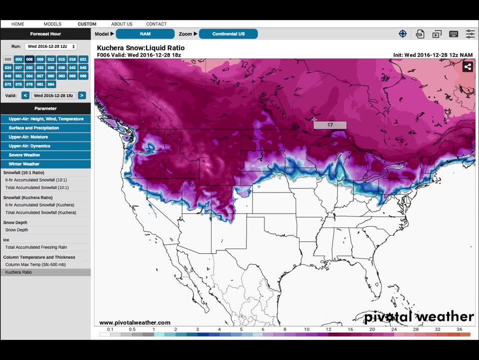 There was snow up here we were examining. We'll say it's a 17 to 1 ratio. That means, if we'll say 0.1 inches of liquid fall, that QPF- we were talking about quantitative precipitation- If 0.1 inches of liquid falls, that means 1.7 inches of snow will fall because it's 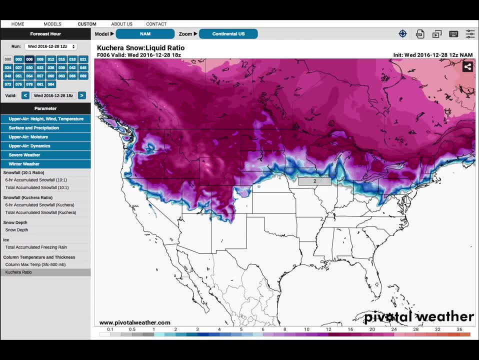 a 17 to 1 ratio. That's good. Down here it's a 2 to 1 ratio. Down here it's below that because it's probably not going to snow down there. It's probably about freezing, But anyway, that's what that is. 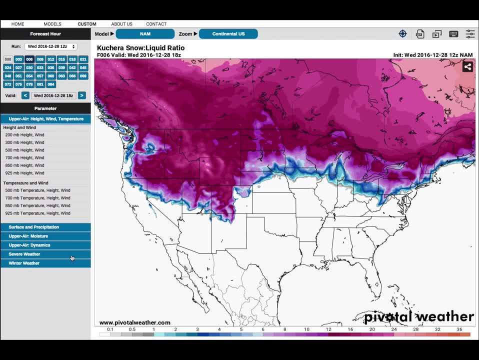 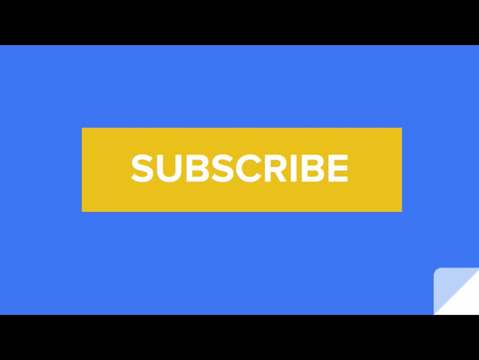 Those are all of your sections that you can examine all your little parameters there. That being said, if you want to supercharge your forecasting skills and you want more weather forecasting tutorials and forecasting breakdowns, where I'll actually show you those models while we're at it. 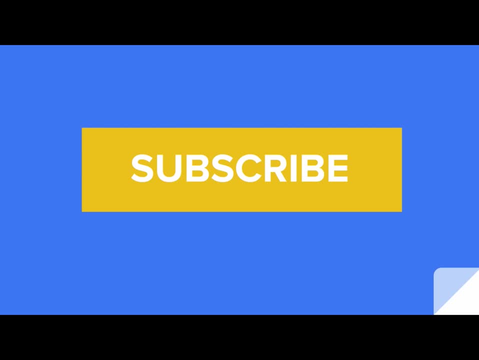 I'm going to show you some of those. I'm going to show you some of those. I'm going to show you some of those. While we're forecasting actual weather week to week, go and click the subscribe button here in the middle of the video, here, and I'll be releasing more forecasting tutorials and. 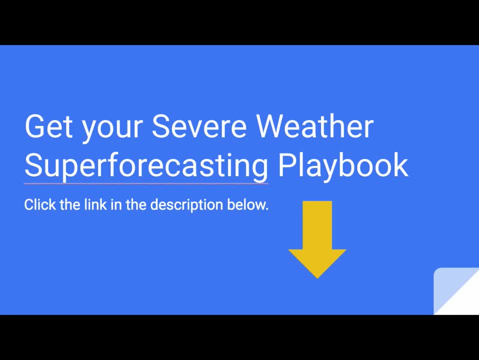 forecasting breakdowns Also, if you're interested, I actually made a book called the Severe Weather Super Forecasting Playbook. It's essentially a cheat sheet guide for forecasting different types of severe weather, hazard types, whether it would be tornadoes or not. 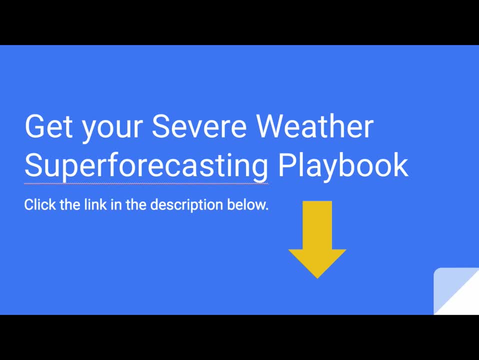 There's like checklists in there. It's essentially like a playbook. If you want that book, hey, I put it in the link in the description. Just click the link, enter your name and your email and I'll send it right off to you. 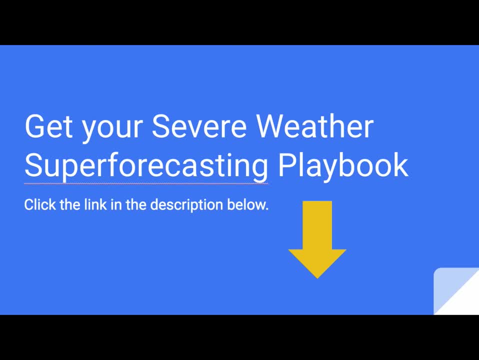 I'll also send you some other updates as well, like some other forecasting tutorials and forecasting breakdowns, some exclusive ones. Go ahead and do that. If you want that, go and subscribe. Hope you enjoyed today's video. If you have any topic requests, go ahead and comment in the video. 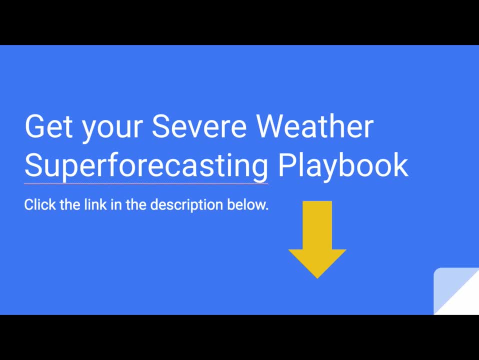 I'll continue to make some more forecasting tutorials based off your feedback. Hope you enjoyed the video and I'll see you soon. 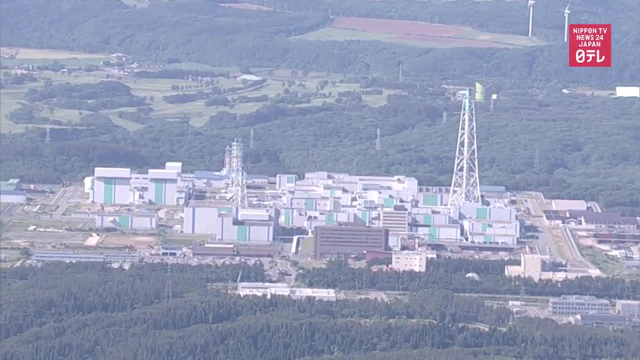 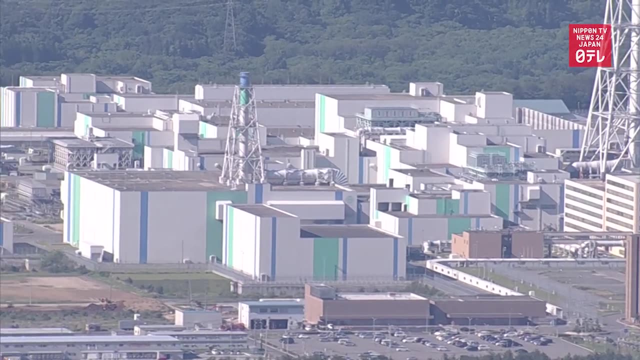 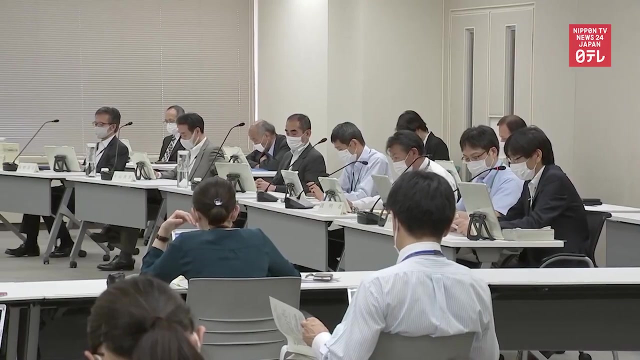 The Nuclear Regulation Authority approved on Wednesday the safety inspection document for a nuclear fuel reprocessing plant in Rokasho, Aomori Prefecture. Officials say the plant meets the new safety standards adopted after a 2011 Great East Japan earthquake. The approval is expected to be finalized after a one-month period of